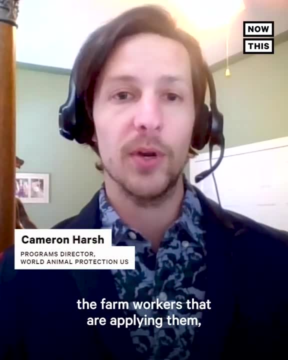 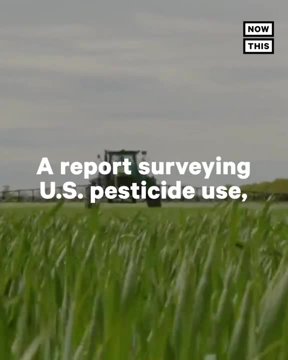 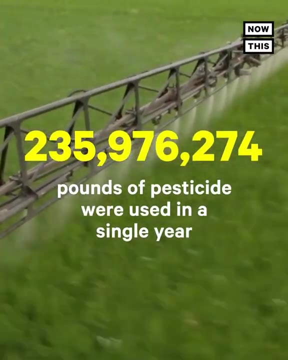 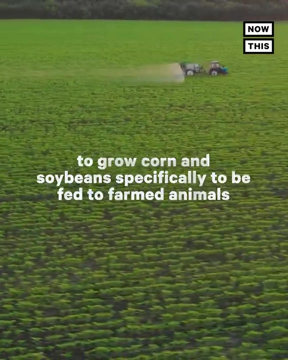 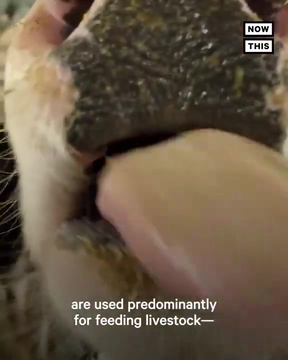 sprayed simultaneously that are impacting wild animals, the farm workers that are applying them, the health of our waterways and ecosystems. Very little of our soy in the US is going directly to human food consumption. Corn and soy grown in the US are used predominantly for feeding livestock. 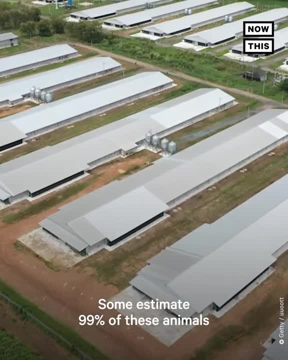 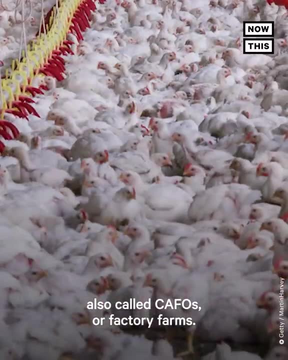 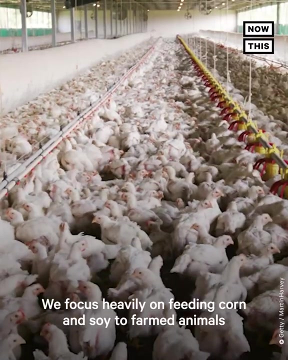 The farmed animals that produce our meat and dairy. some estimate 99% of these animals are in confined animal feeding operations, also called CAFOs or factory farms, and those animals are being fed billions of pounds of predominantly just two crops: corn and soy. We focus heavily 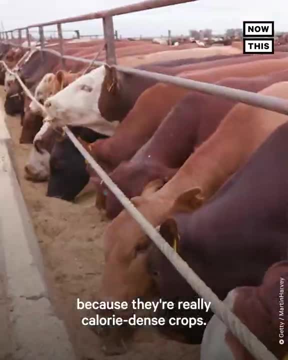 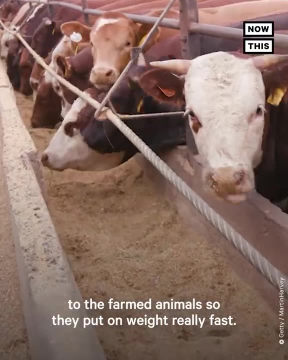 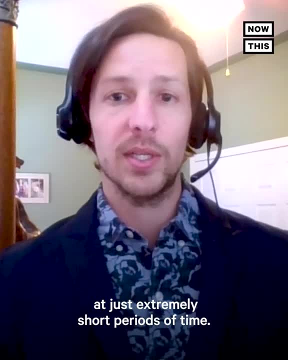 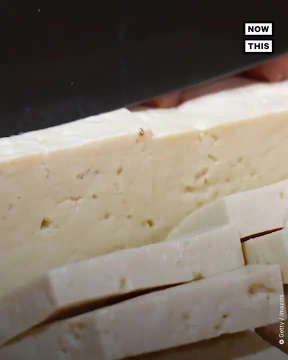 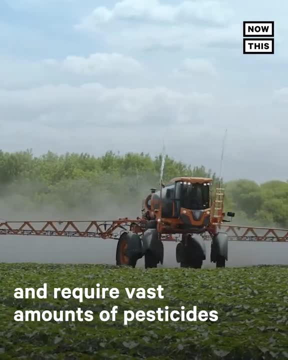 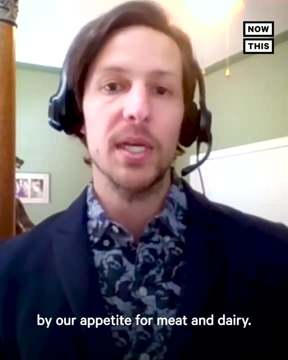 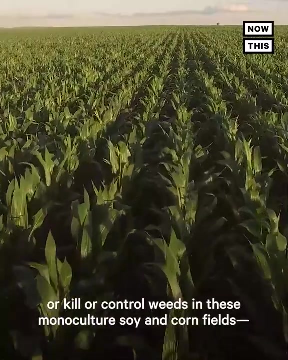 Wild animals are directly impacted by our appetite for meat and dairy. The pesticides that we're using to kill or control insects or kill or control weeds in these monoculture soy and corn fields, chemicals like glyphosate and atrazine, and neonicotinoids. 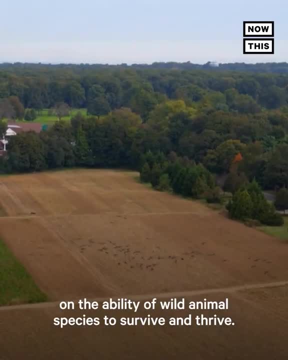 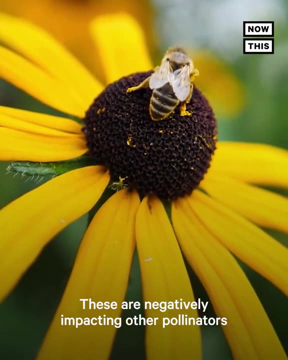 they are toxic chemicals that are having an impact on the ability of wild animal species to survive and thrive. These are negatively impacting other pollinators like bees, and particularly native bee species that we rely on for pollinating the foods that we need to eat. 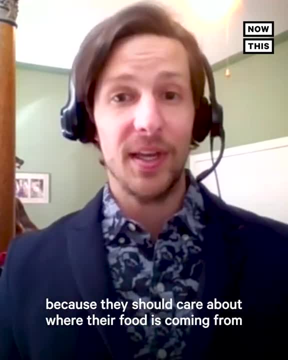 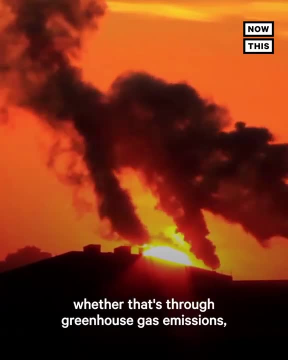 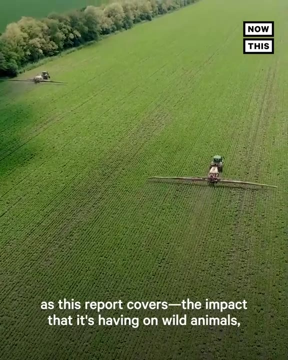 The average person should care about this issue, because they should care about where their food is coming from and the impact that their food is having on the planet, whether that's through greenhouse gas emissions, the impact that it's having on the climate through pesticide use, as this report covers, the impact that it's having on wild animals.